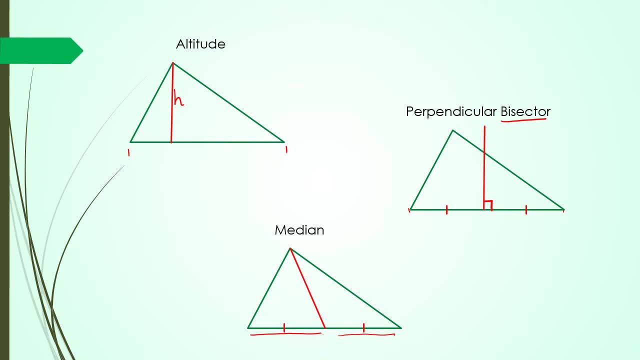 bisector is going to look like okay. so yes, there can be situations where you could potentially get altitude, median and perpendicular bisector all in the same line. I think that's if you work with an isosceles triangle, with a 45 degree isosceles triangle, you'll end up with that. but that's for later, so right. 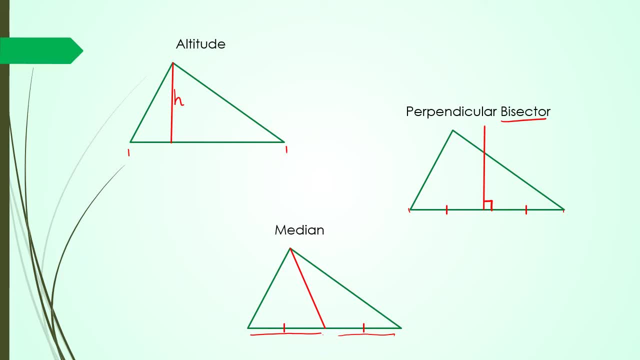 now remember that you have three properties. altitude is the height, median is from the vertex of the cone, from the vertex to the midpoint of the other line, and then for the perpendicular bisector, it's basically a line going through the midpoint at a perpendicular. as a perpendicular line, that's going through the midpoint. cool, let's have a look at some questions. 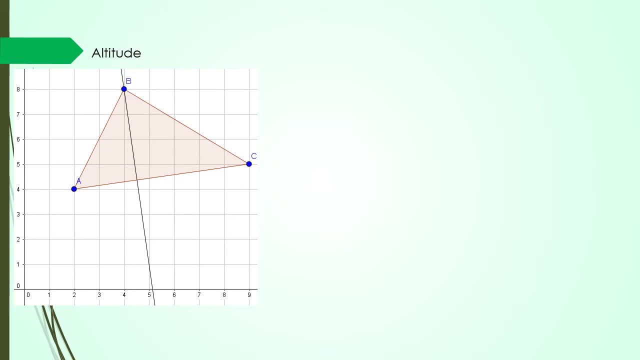 so in this question i would like to find what am i looking for. i'm actually looking for the altitude, all right, so i know it's the altitude, because i can kind of see that it's not really in the middle, so it's not a perpendicular bisector, nor is it a median. so how am i going? 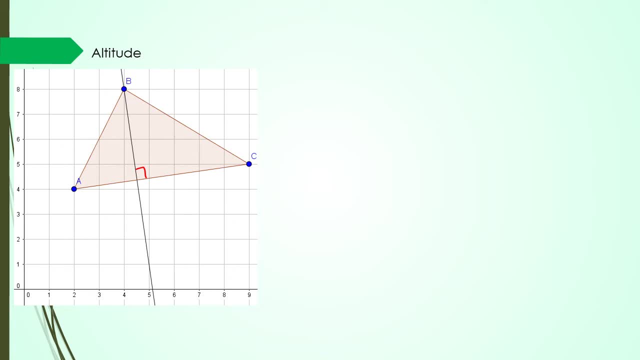 to work out the altitude in this case. now let me do the first thing. i'm going to call this point d here. so how am i going to find the altitude? when i say how am i going to find the altitude, i'm actually looking for the equation of the altitude. all right, so to get started to find the equation. 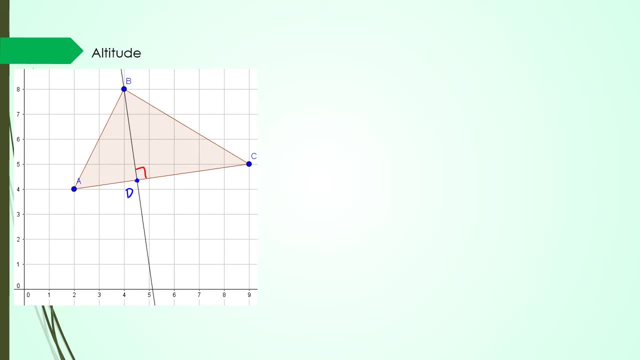 of the altitude. what i'm going to need is i'm going to need a gradient. all right, i'm going to need a gradient and i've got a point which is b, so that's fine. so first thing i'm going to do is i'm going to work out what gradient of ac is. 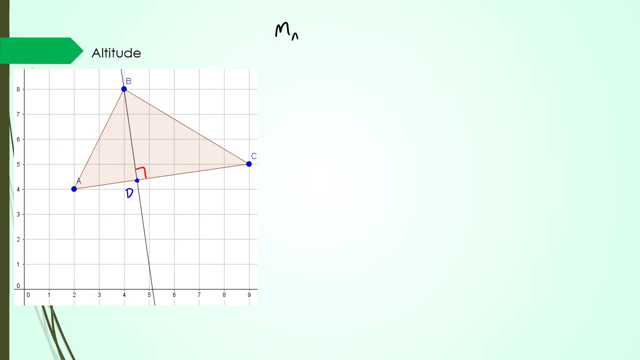 so i'm going to work out a gradient of ac. so that's y2 minus y1 over x2 minus x1. now, looking at the points i've got, here are 9, 5 and in this side i've got 2- 4. so my gradient is going to be: 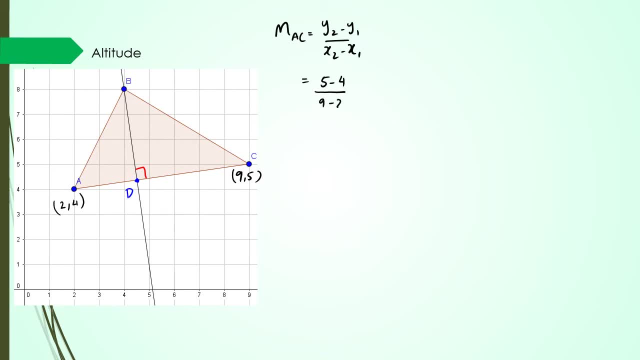 5 minus 4 divided by 9 minus 2, so my gradient is 1 over 7. so because ac's gradient is 1 over 7, now to find the perpendicular lines, which is bd. so gradient of the bd equals negative 1 over gradient of ac. so i'm going to have negative 1. 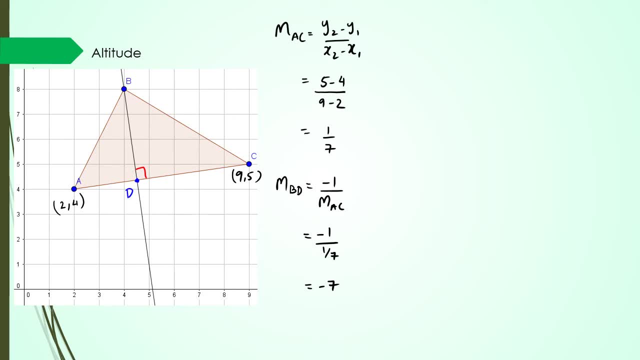 divided by 1 over 7, which means the gradient is equal to negative 7. now i already have point b, which happens to be 4- 8, so i can actually work out the equation of the altitude in this situation, because my gradient of bd equals negative 7 and i'm going to use point b, which is 4- 8, so putting this all in an equation. 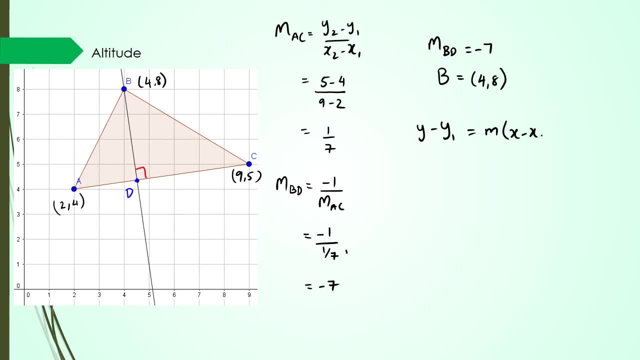 this is equation of a line. so y minus 8 equals negative 7 times x minus 4. i've got y minus 8 equals negative 7 x plus 28. so this is the equation of the altitude in this for this particular question. next i'm going to 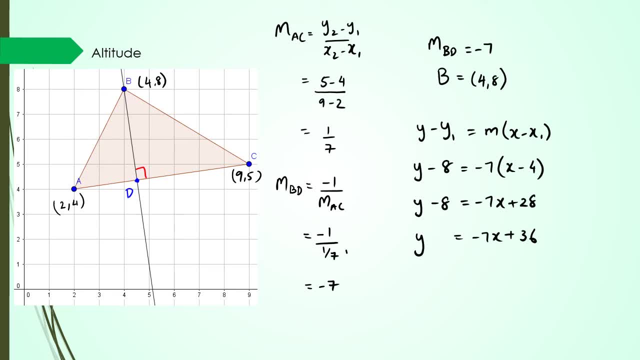 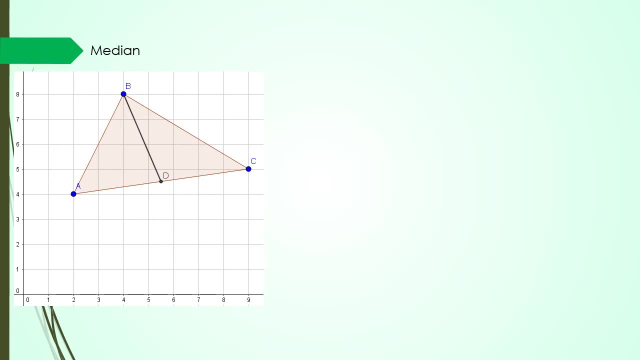 show you guys how to work out. well, i don't know which one is popping up, but whatever it is, we'll work through it, all right. so in this one, it looks like we're going to work out the equation of the median. all right. so i'm going to show you guys how to work out the equation of the median. 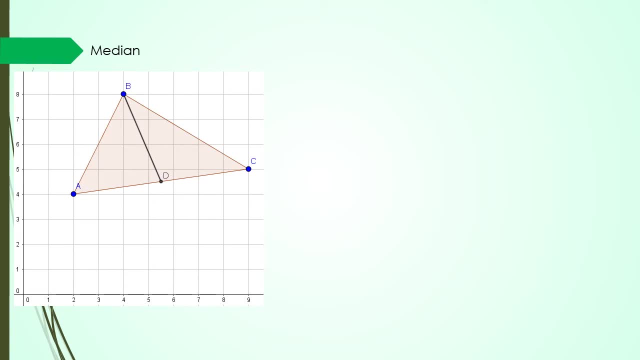 all right. so now i'm going to use the same triangle guys, just to make things a little bit easier here. all right, so i already worked out what the gradient of ac was from the previous question. so gradient of ac equals negative, uh, one over, uh, sorry, positive one over seven. but is the gradient going to be any use in here? well, 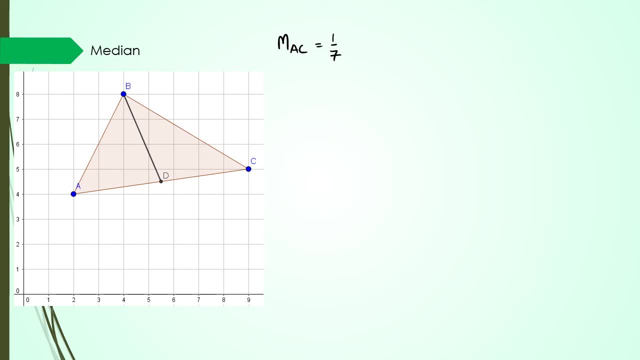 it's not for starters, this is not a perpendicular line, so i don't really need a gradient of ac in this case, so i'm going to use the same triangle, guys, just to make things a little bit easier here. but what i do need is i need point d. all right, and point d is the midpoint between a and c. 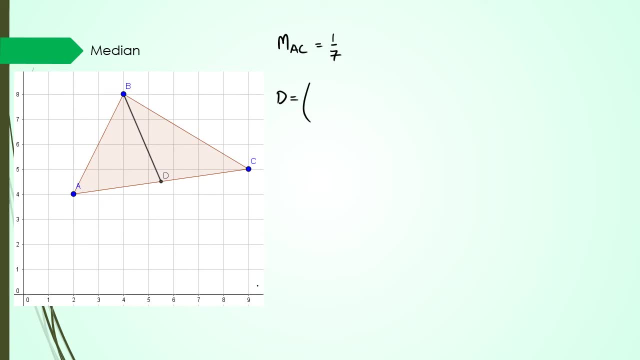 so to work out point d, i've got x1 plus x2 over 2, y1 plus y2 over 2. now my two points: as usual, i've got c as 9 and 5, a as 2 and positive 4. so putting this together i would have: 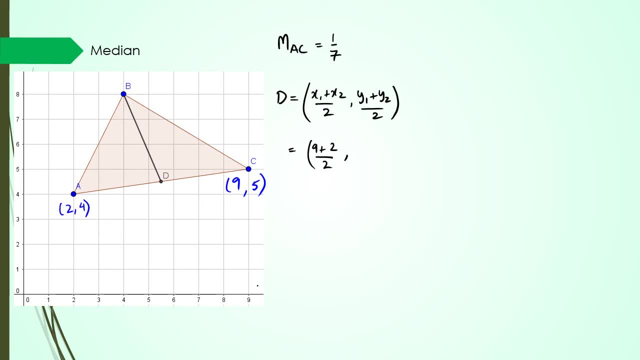 9 plus 2 divided by 2 and 5 plus 4 divided by 2, which means i've got the points 5.5 and 4.5 as the point d. now i also have point b. point b is 4 and 8. 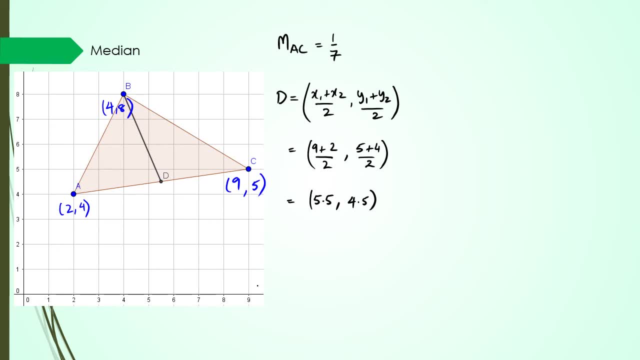 so at the moment i've got point d and i've got point b, so i need to work out gradient of bd. once i get gradient of bd i can use one of the points to substitute and find the equation of the line. so i'm going to 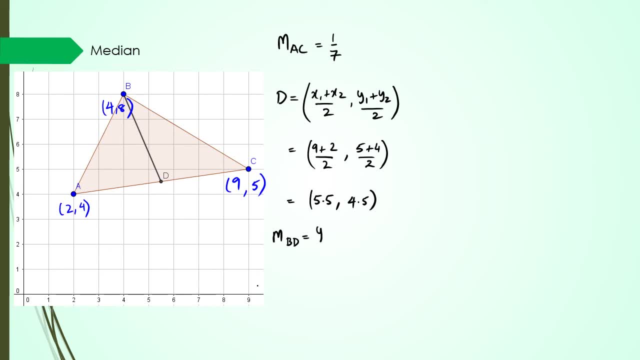 find gradient of bd, so that's y2 minus y1 over x2 minus x1, now y2. in this case i'm going to use 8 minus 4.5, divided by 4 minus 5.5, which means i have 3.5 divided by negative 1.5. 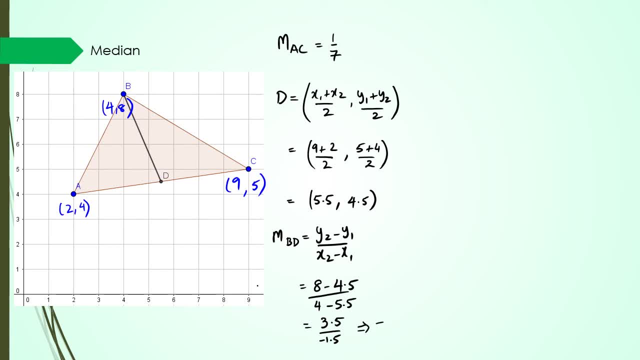 now i'm going to simplify that to negative 7 over 3, so that's just a nice number to work with for me. all right. so i've got the gradient of bd and i'm trying to work out the median, which is bd in this case. i'm trying to work out what the equation of that line is. so i've got my gradient, which is. 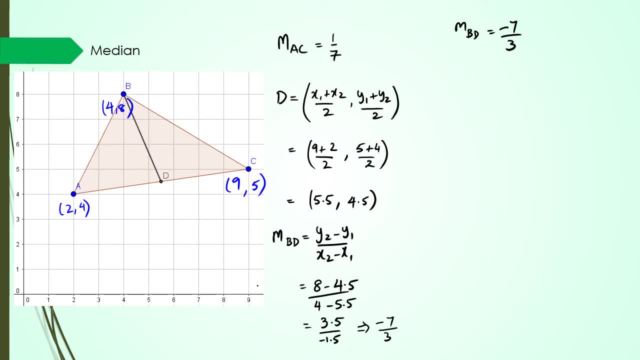 gradient of bd equals negative 7 over 3, and then i've got a point which i'm going to use, which is I'm going to use 4- 8. so therefore I can put this as my equation: well, not y2, sorry, y minus y1. 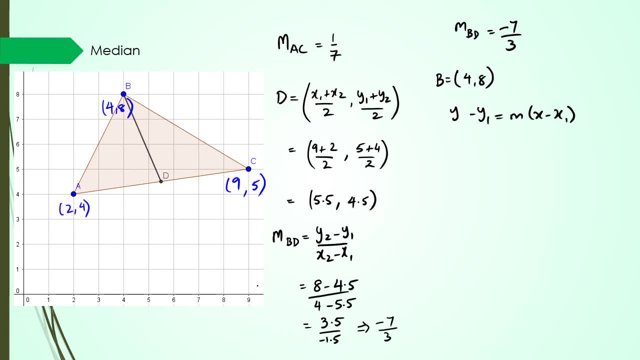 equals m times x minus x1. so I've got y minus 8 equals negative 7 over 3, x minus 4, and I have y equals negative 7x over 3 plus 28 over 3, and then, rearranging this, I would have 28 over 3. 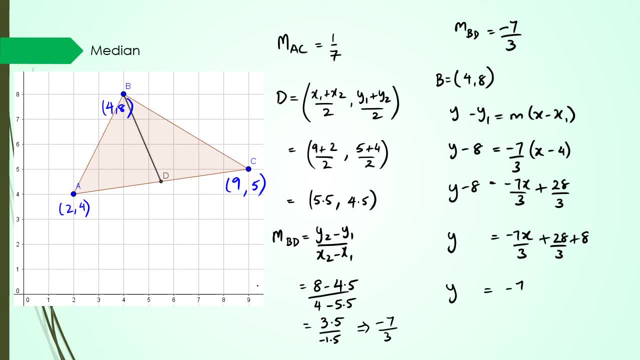 plus 8. simplifying this further, I should have 28, 24, 24 and 28 is going to be 22, 52 over 3. okay, so that's the equation for the median in this case. so we can actually say: equation of bd equals negative 7 over. 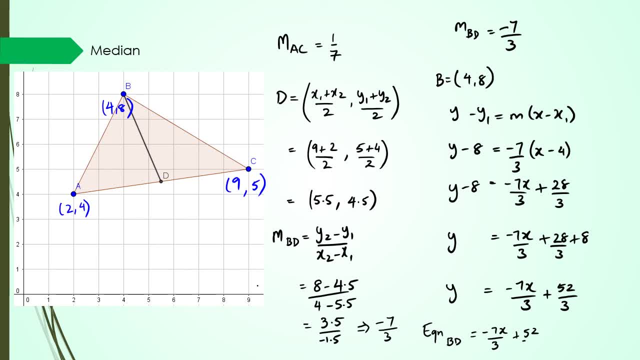 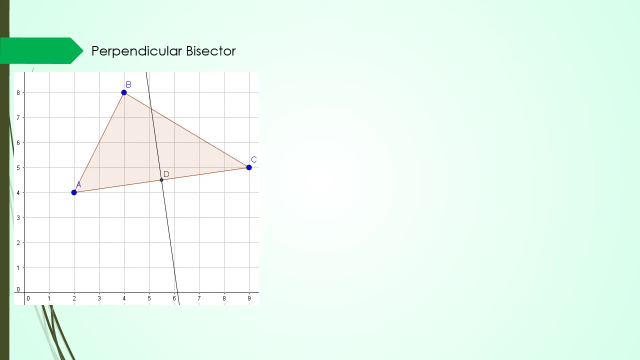 negative 7x over 3 plus 52 over 3. okay, so the next one I'm going to be looking at, perpendicular bisector guys. so what do we know from here? and I guess with this one we kind of we kind of need a gradient of ac. 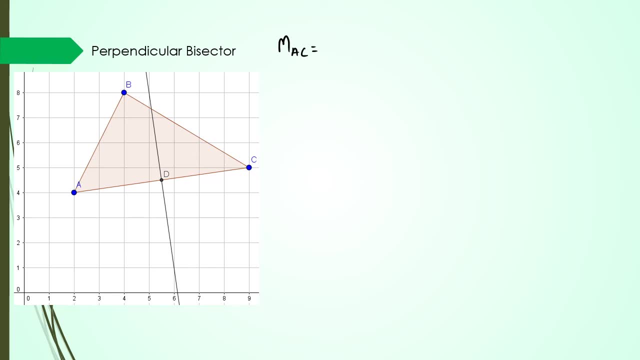 so, which we already have from the first slide, gradient of ac equals to positive 1 over 7. we also know what point d is from the previous question that we did. so point d was 5.5 and 4.5. so the equation for the perpendicular bisector is just using these things. so I've 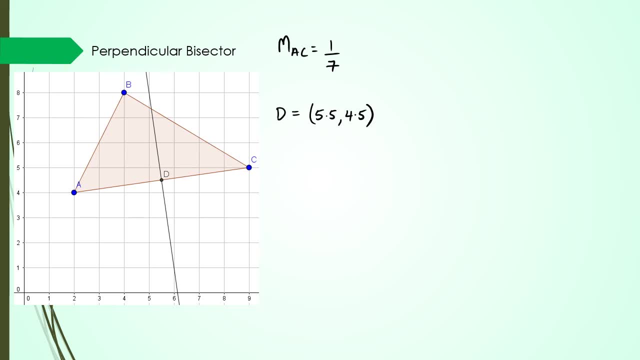 got the gradient. oh no, sorry, I need gradient, the perpendicular gradient. so what you can write is: let's see this perpendicular gradient for ac. actually write it like: this is negative 1 over 1 over 7, which means negative 7. all right, so I've got the perpendicular. 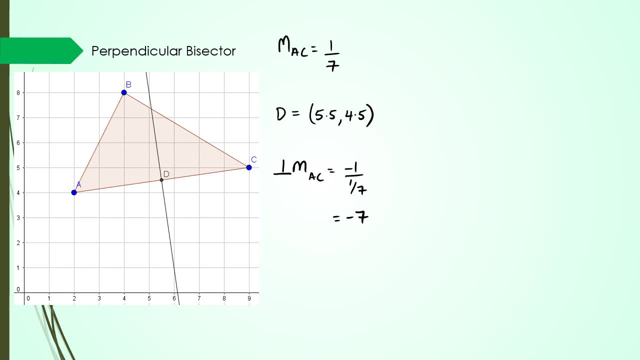 gradient which is negative 7. that's this black line here. now it's just constructing the equation. so I've got y minus y1 equals m times x minus x1, and I already have my points, which is 4.5 and 5.5.. Gradient is negative 7x minus 5.5. So 4.5, we've got negative 7x. 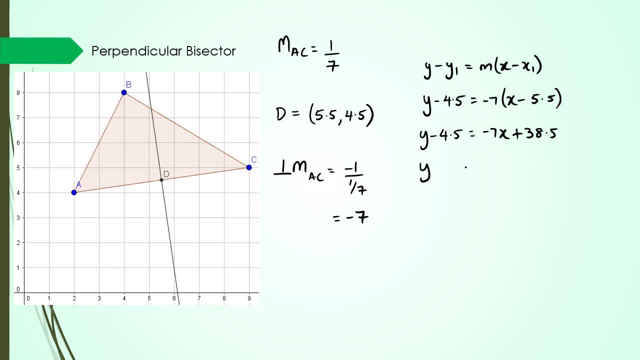 plus 38.5.. And then y equals negative 7x plus 38.5 plus 4.5.. And so the equation for the perpendicular bisector is going to be negative 7x plus 43.. Okay, so that's basically it for this. 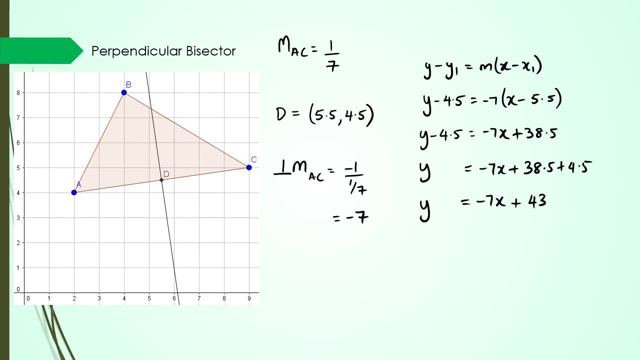 session, guys. So we've covered three things here: altitude, median and perpendicular bisector- And this is working with triangle properties. Okay, that's it for this session, folks. If you have any questions, pop it in the comments and I'll try and get back to you. All right? thanks for watching guys.